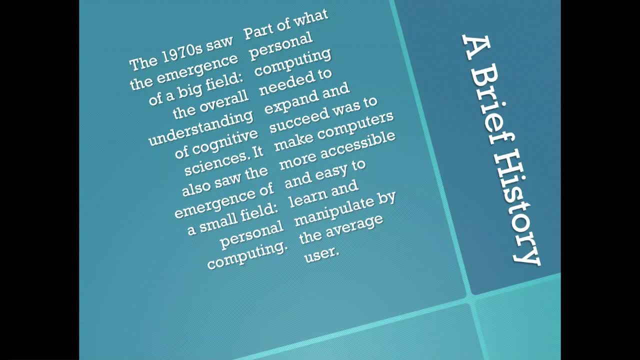 that may mean. In response to this emergence, the field and use of the term human-computer interaction developed. At this same point in time, many different fields of science had begun to merge under the heading of cognitive science, A big part of which was the idea of cognitive engineering. 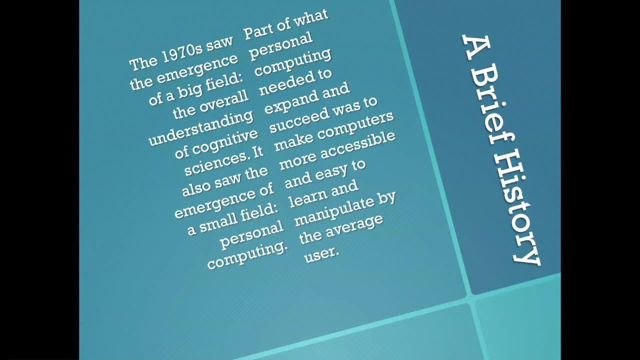 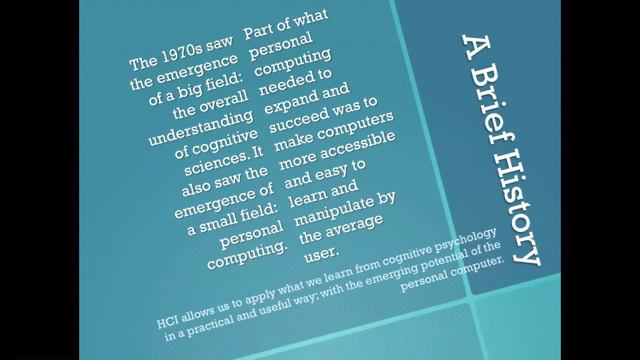 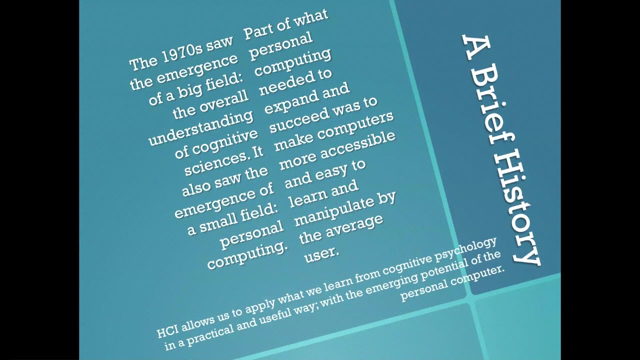 looking at the mental and motor processes of humans and how they influence and are influenced by our interactions with people and objects. So, just as the need for HCI arose with the arrival of personal computing, the field of cognitive science arose with the ideas and concepts that HCI needed. HCI was to become 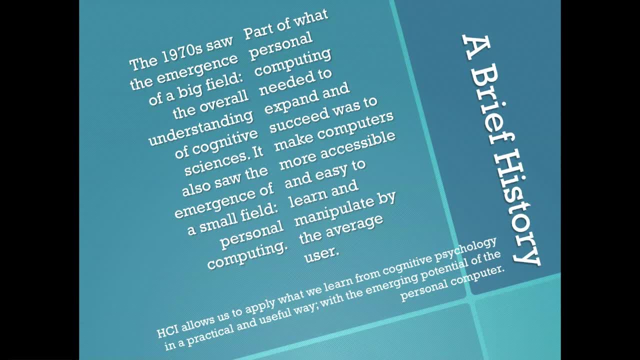 one of the first examples of human-computer interaction. HCI was to become one of the first examples of human-computer interaction. HCI was to become one of the first examples of cognitive engineering and was, and still is, a bold merging of science and engineering. 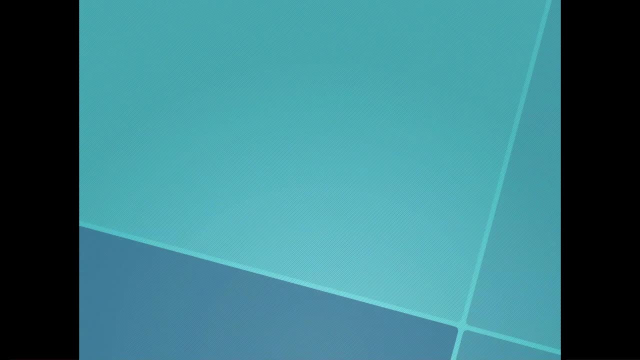 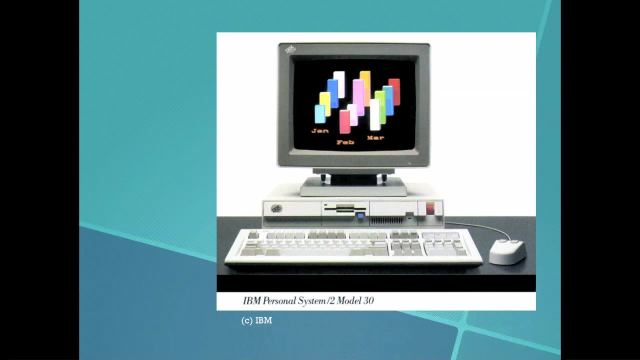 Let's take a look at some of the first examples where the ideas of HCI were to be applied. Before personal computers such as this IBM, the main computer output was text on a screen and the only input a keyboard, While this is still a common input-output paradigm used. 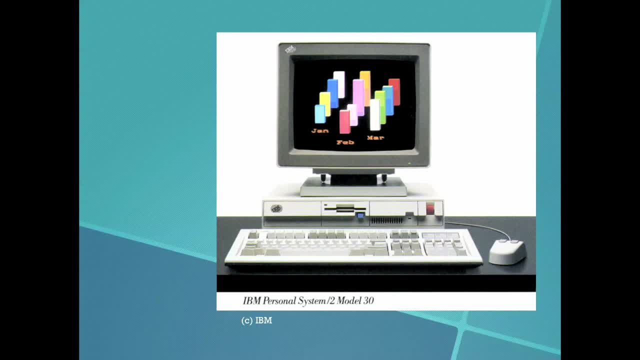 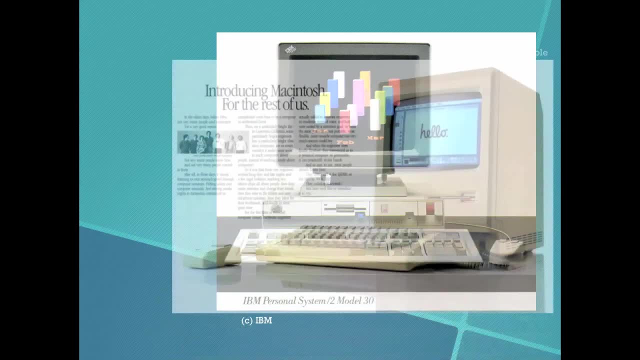 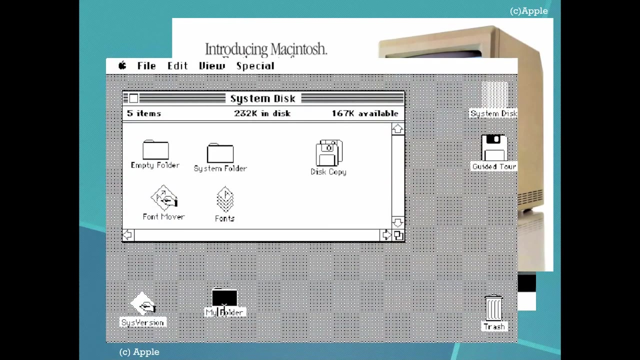 today. it was hard for the casual user at first and as the only means of interacting was less than intuitive. QHCI and the invention of the mouse and the development of the cluttered desktop design. Using the mouse, the desktop became a clear space where users could move, organize, hide. 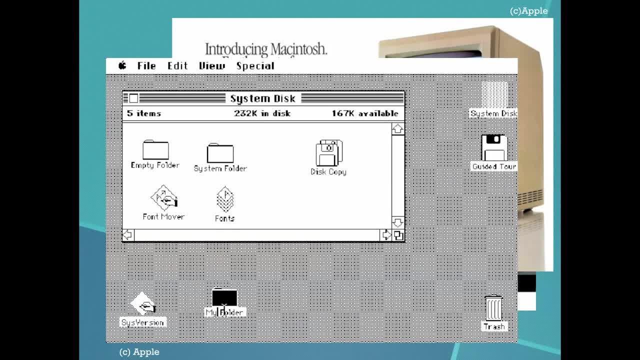 delete and often lose files and documents very much like they would with physical documents on a physical desk. It was a simple, relatable and intuitive way of displaying digital information and caught on extremely quickly, still used to this day When the desktop first developed. 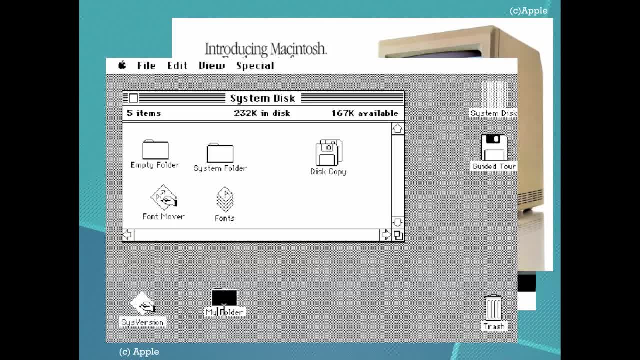 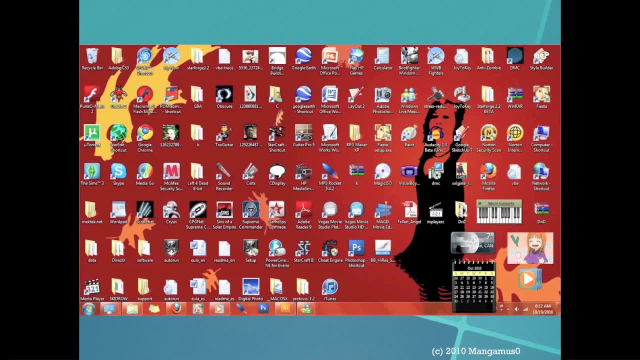 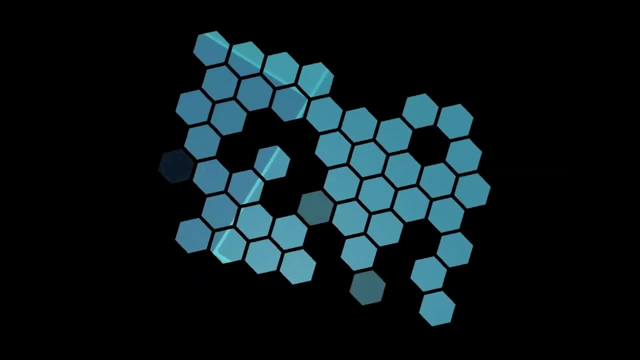 it was revolutionary and exciting. But as our world evolved and as the amount of digital information exploded, the cluttered desktop idea started to lose some of its initial magic and usability. Thankfully, the study of HCI hasn't stood still. The desktop is no longer the central key to our interactions with technology. With the 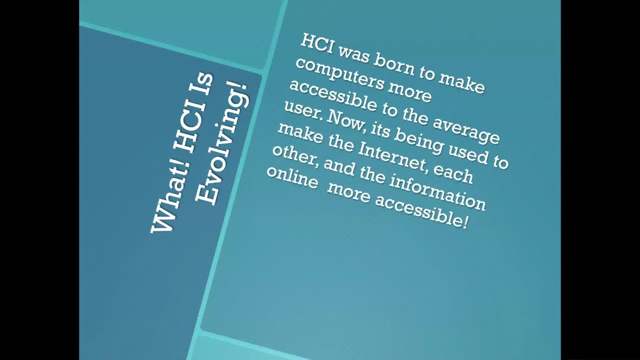 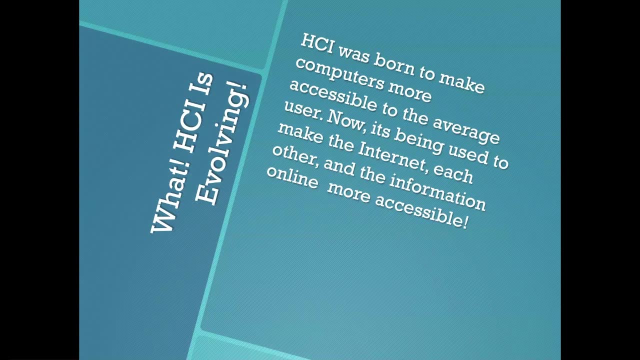 rapid expansion of the web, the variety of technologies used to connect people and things in every part of the world has also expanded. The web browser has become as much our homepage as the desktop once was. The ideas of HCI have paved the way for social networks, blogs, email systems and instant text and video. 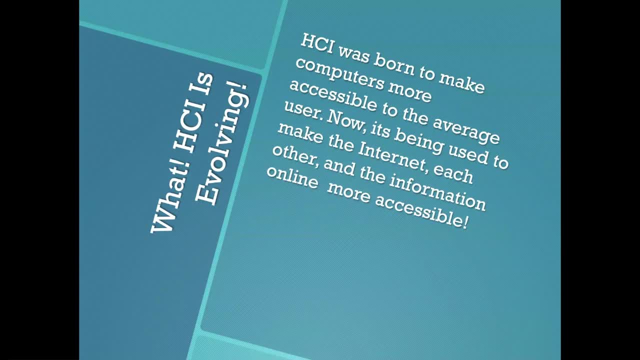 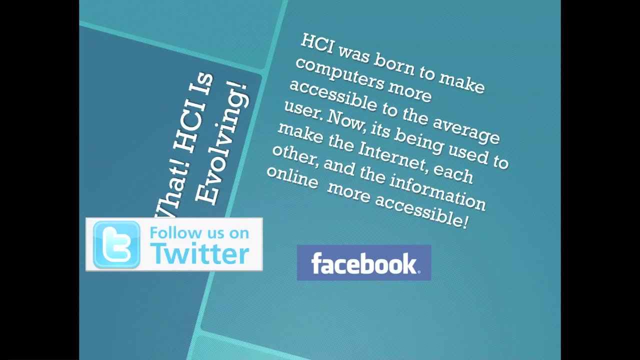 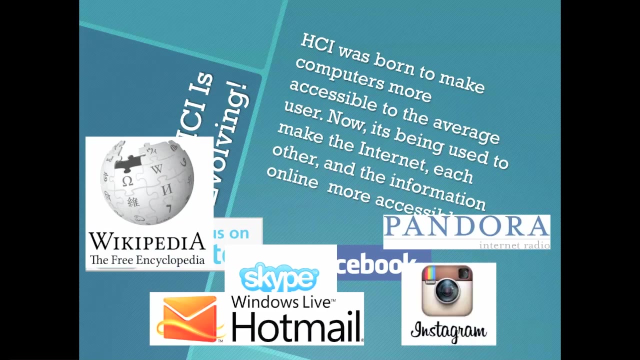 chat programs to become seamless parts of our daily lives. The brisk, clean interfaces and free-to-use nature of services like Facebook, Twitter, Skype and Gmail have opened unprecedented levels of communication between users and their systems. It is largely through the inspiration 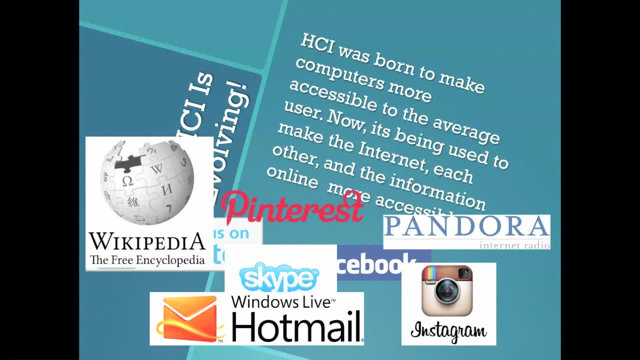 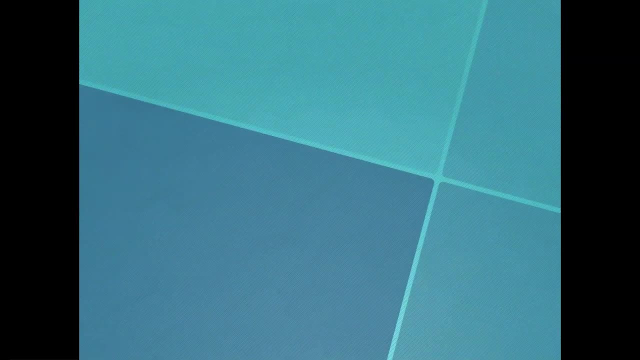 and popularization of HCI, that the desktop has become a place where users can access and share their content. HCI includes all the ideas we learned about the TEDS Value Added Model. TEDS provides clear guidelines on how to make a system accessible on an editable top-layer level, such as clarity. 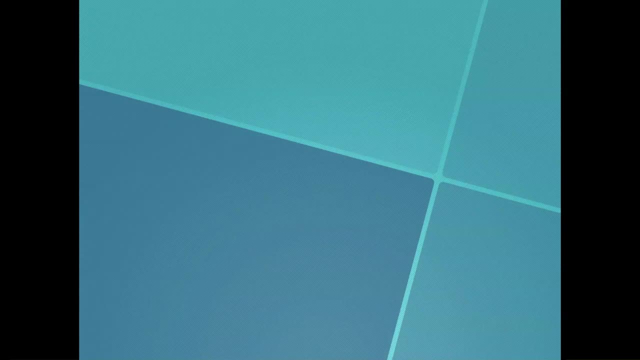 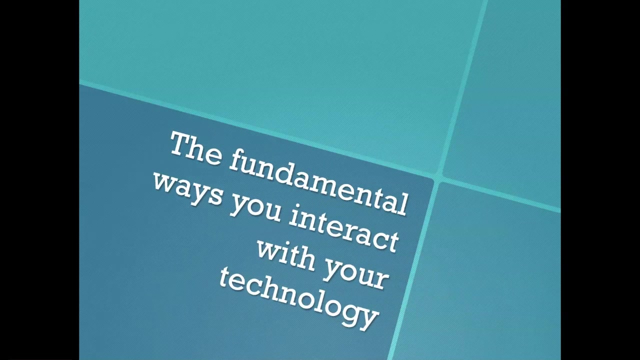 of links, aesthetics and overall smarts of a system. HCI includes this, but goes much deeper, focusing as well on the most fundamental ways we interact with technology and systems. Some of the advantages of HCI in practice are everywhere you look from the open, customizable. 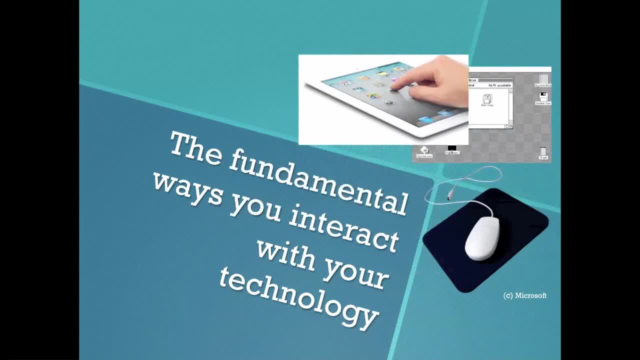 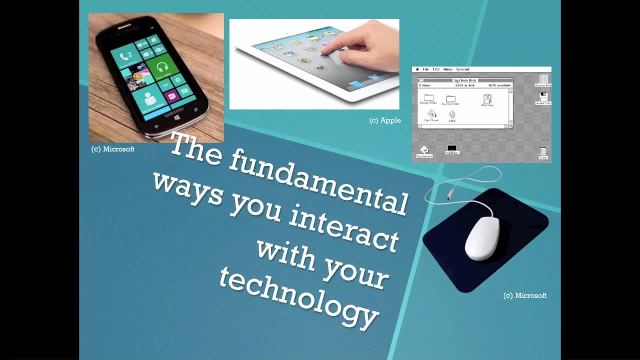 nature of a desktop to the simple, minimally customizable interface of an iPad. Even within specific arenas, there are widely differing offers. Smartphones are a great example. Microsoft and Apple have both implemented systems with simplicity and ease of use in mind, allowing 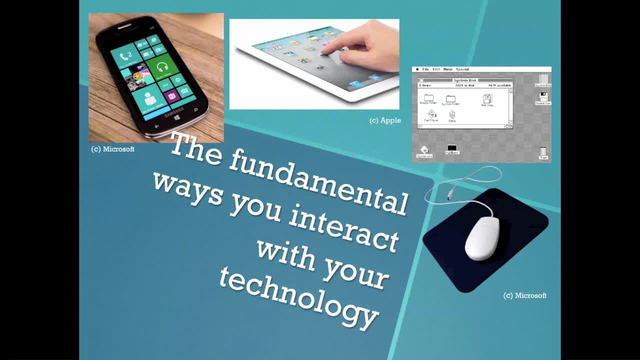 little customizability. While one of the core design principles behind Google's MOLO OS is the idea of open-source and customizability, Microsoft, Apple and redesigned software have both implemented systems with simplicity and ease-of-use in mind. Today, everyone involved in a technology is a part of that custom. 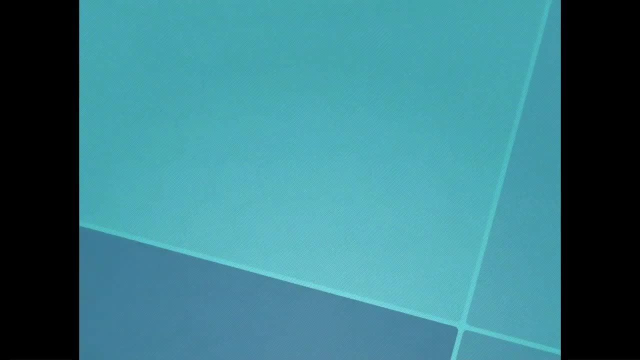 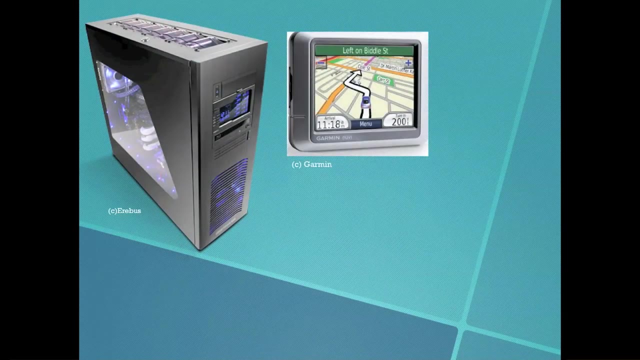 and both are able to utilize the technology at all times And at least 100% of the customers have a technology field has HCI in mind, though to varying degrees of success, of course, From the manufacturers of PC hardware to the animations behind vehicle GPS systems and the technicians. 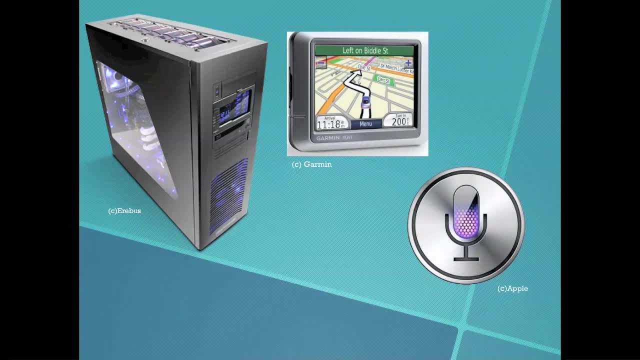 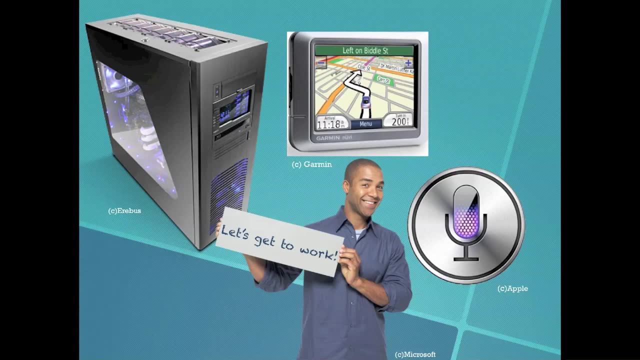 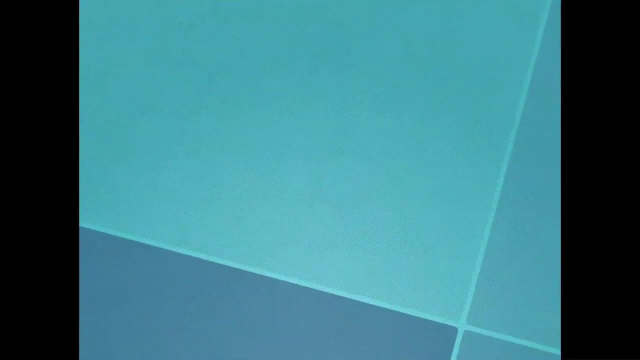 who created the exact tone of Siri's voice. Technology is used by people, and every change, improvement or innovation in technology is inevitably related to how people interact with that technology. As our needs evolve, so does technology and the ways in which it can help us. 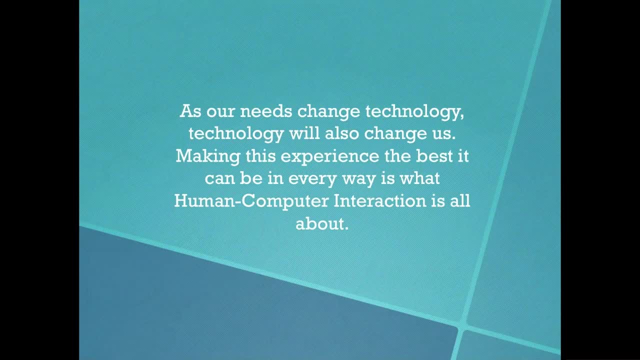 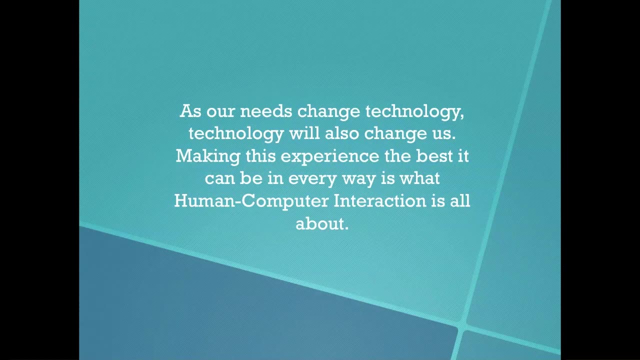 meet those needs. HCI is right there, at the forefront, expanding and evolving along with it, always making sure that, as new technologies develop, we don't lose sight of that key idea: designing systems with a focus on usability, making it easy to use, easy to learn.